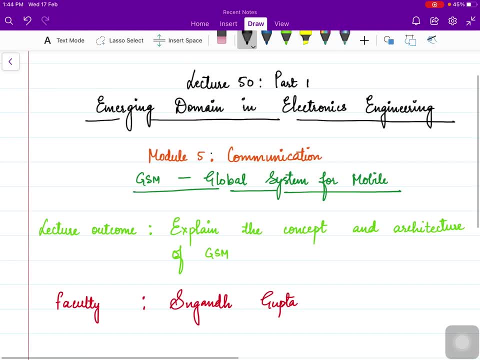 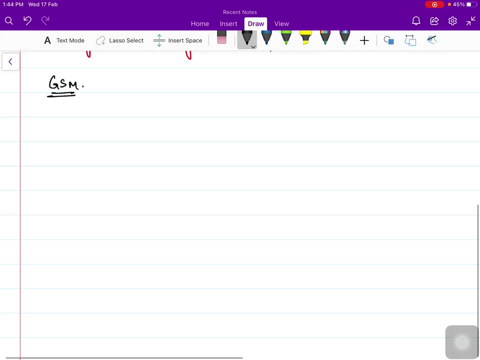 GSM. So let us see the architecture of GSM first. So the architecture of GSM is: we have mobile stations, several mobile stations. Mobile stations is nothing but the handset that we are having. So multiple users are having multiple mobile stations. So mobile station is nothing but your mobile handsets And they. 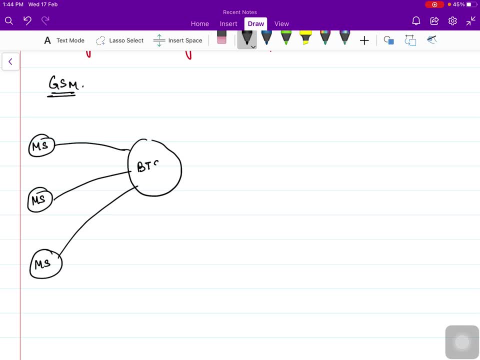 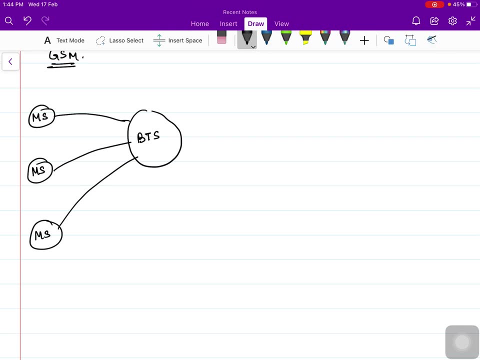 to the base trans receiver station. base trans receiver station, that means which transmits and receives. so this BTS is nothing but the towers that we see outside our homes, so like Airtel tower, Vodafone tower, so the towers which we talk about, that today the signals are weak, or today? 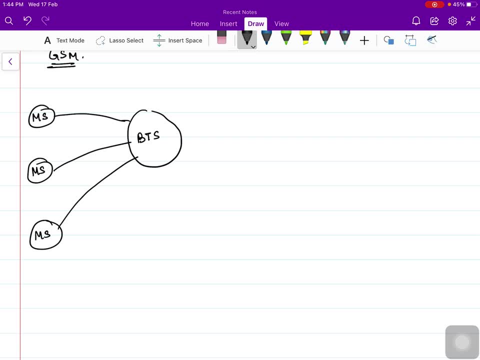 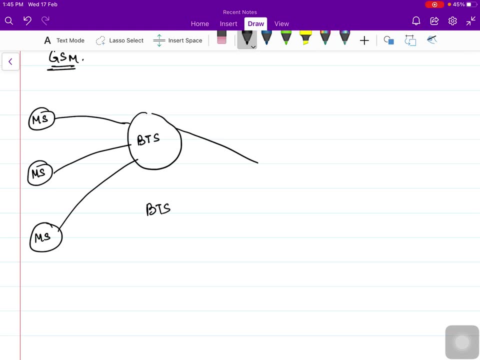 the signals are strong, so they are provided by this BTS, okay, and the one which controls the BTS- now, there are several BTS- and the one which controls the BTS, all the BTS, that means, which looks for the coordinating these towers, which looks for the maintain, looks after the maintenance. 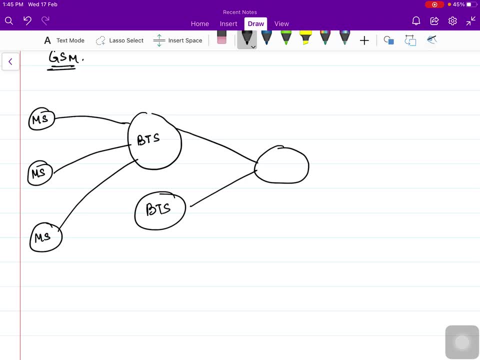 of these towers, that is BTS, which looks for the facilitating these BTS. okay, so that's nothing but base station controller. so we frequently talk that today the signals are weak or strong, so that are controlled by BSC. okay, towers are BTS. there are multiple BTS and the one which controls the towers that is BSC, so it is the base station controller. now, every 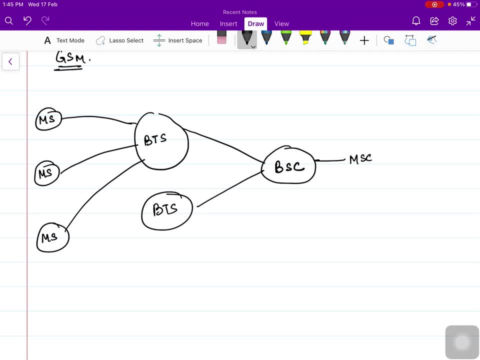 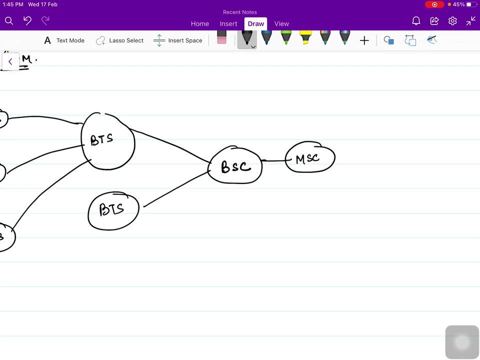 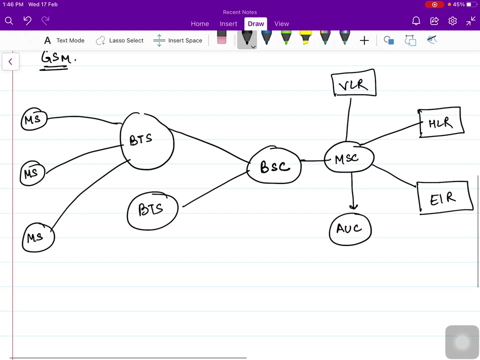 base station controller. it's connected to MSC. that is mobile switching center. okay, and the mobile switching Center is connected to AUC, VLR, HLR, EIR, so that is MSC. MSC is connected to these devices. So this part, you can say that this basic structure of the 74 part, fingerprints and batters are 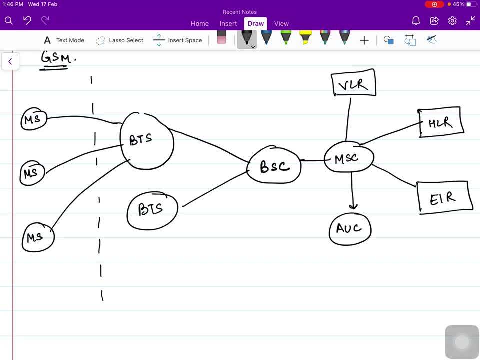 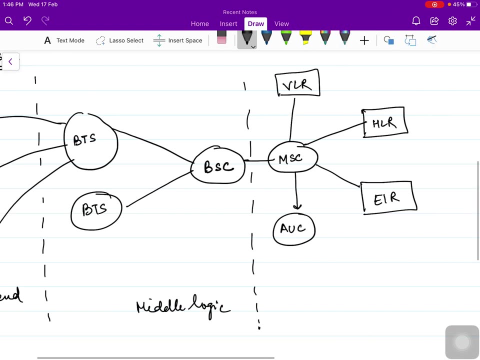 connected to counter income rate, then you can use data. the manufacturers and manufacturers make the fish problem highly broken and you briefly will explain in a later video you can see on the displayed screen. This is the front end, this is the middle logic and this is the back end. 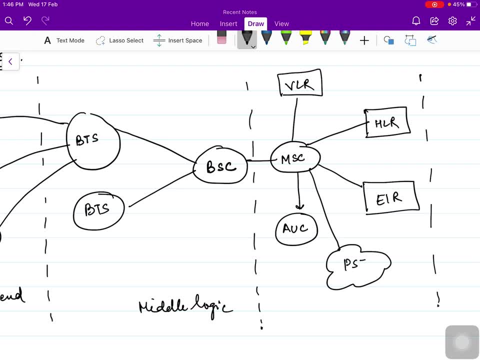 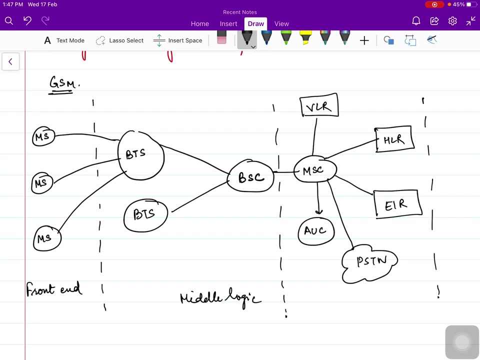 This is also connected to PSTN, Public Switch Telephone Network. AUC stands for Authentication Centre, EIR stands for Equipment Identity Register, HLR for Home Location Register, VLR stands for Visitor Location Register. So these are the registers with the help of which MSC, that is, the Mobile Switching Centre, 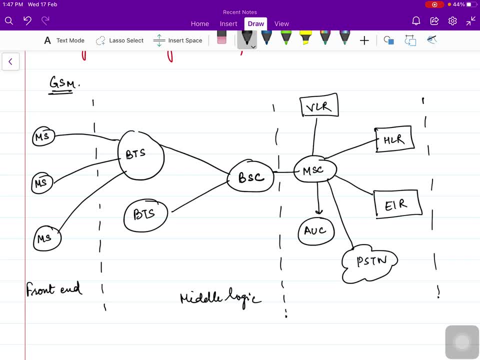 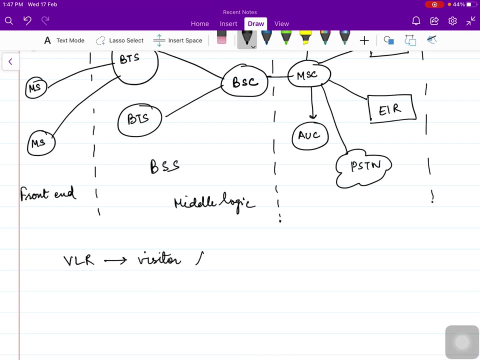 takes care of BSE, that is, the Base Station Controller, and the combination of BSEs and BTS. they are together called as Base Station Subsystem, BSS. Thank you. So what is VLR? VLR is Visitor Location Register, which means it is a database that keeps the record of. 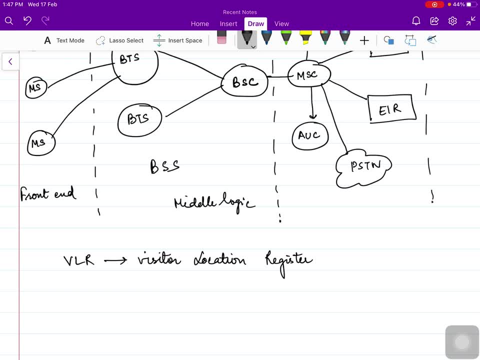 all the subscribers in the network. For example, if one person is moving from one state to another state, so his entry will be marked in VLR. So because it will be entering into the VLR of that- Now HLR, that is the Home Location Register- the person, for example, buys a SIM from Ghaziabad. 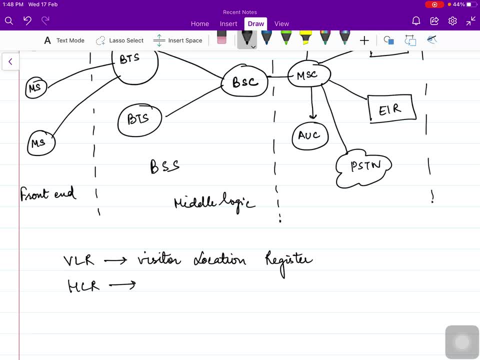 So there will be a Home Location Register for Ghaziabad. So Home Location Register is a database that will keep all the records of the subscriber. That means like the SIM from where he has purchased the place from where he has purchased the SIM. 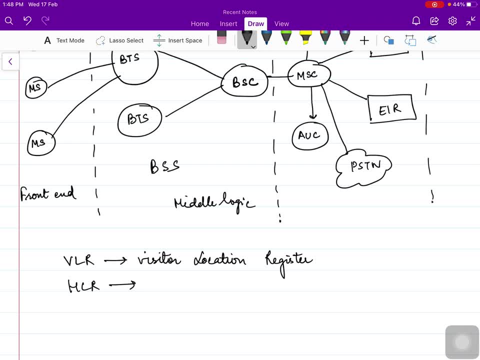 So the ID proofs, that all will be stored in HLR. So that is Home Location Register. It's just like a home. Then the other one is Authentication Center, AUC. That is Authentication Center, So it authenticates the subscriber who has called that. whether the subscriber is authenticated. 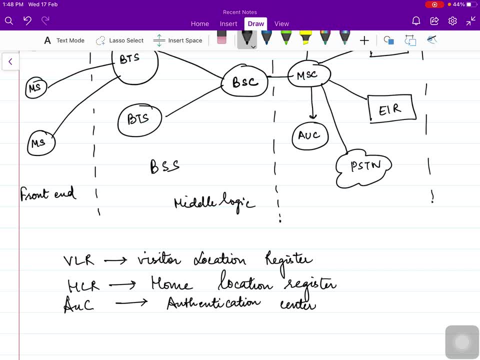 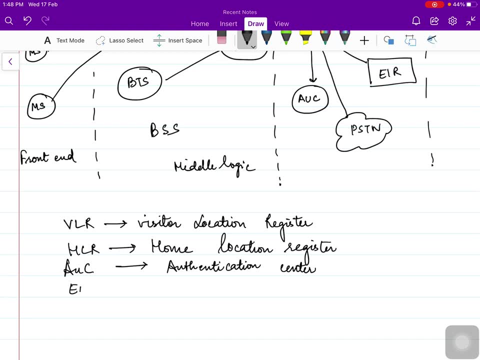 to call in this particular phone Or not. So that is being marked in Authentication Center. Okay, EIR, that is Equipment Register, Equipment Identity Register. It is a database which keeps the record of all the authenticated subscribers or it keeps the record of whether a particular subscriber, whosoever, is banned or whosoever is allowed. 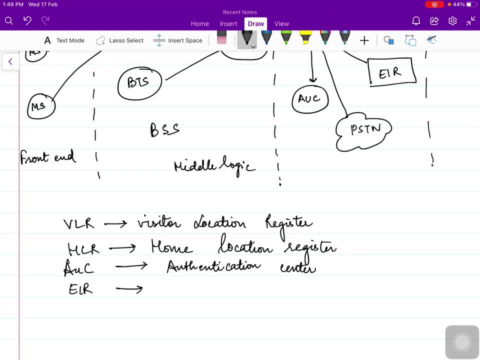 to call in this particular network. So that is Equipment Identity Register. Next one is EIR, So that is EIR. Next one is Equipment Identity Register. Next one is EIR, So that is EIR. So that is EIR. 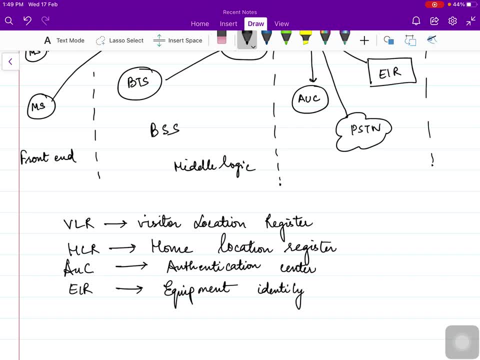 Next one is EIR, Next one is Equipment Identity Register. Next one is Equipment Identity Register. Another one is PSTN, that is, Public Switched Telephone Network. So these are all the parts of the backend and, with the help of all the registers, the 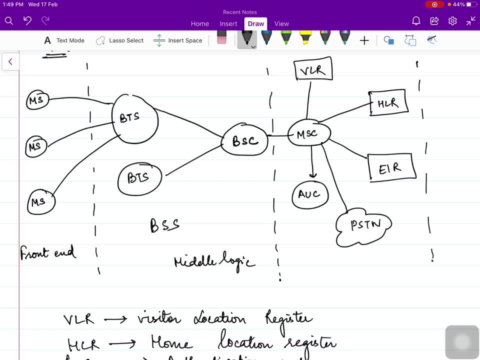 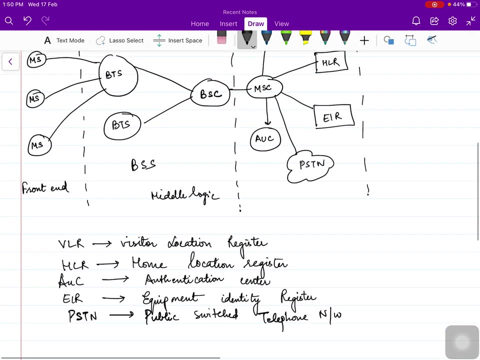 mobile switching center takes control, takes care of BSC and BSC takes care of all the BTS connected to it, and every BTS is connected to multiple mobile stations. So this is the architecture of global system for mobile. Now, if we talk about theory, as global system for mobile is a second generation standard, So 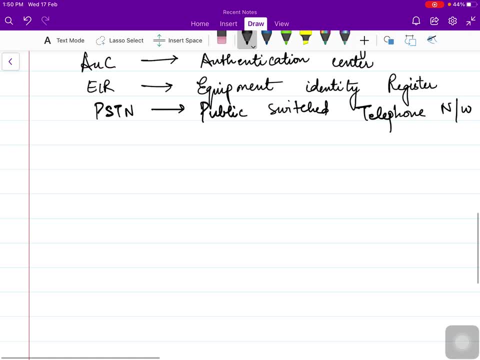 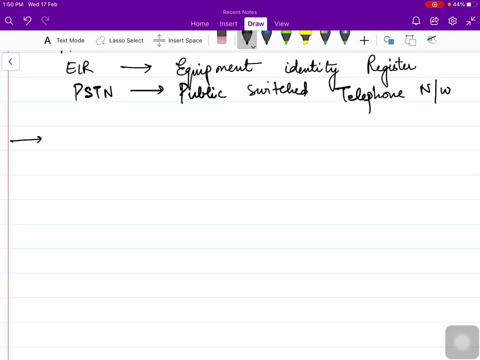 all the features that we have studied in second generation will come in the theory part of GSM. So, basically, what is GSM? It is the global system for mobile communication and it is a standard developed by ETSI. So global system for mobile communication, that is GSM. 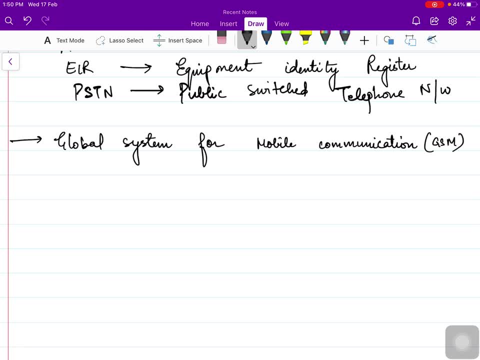 is standard developed by ETSI, that is, European Telecommunication, European Telecommunication Standards Institute, and it describes, to describe the protocols, to describe the protocols. every standard describes the protocols and it describes the protocols for that particular generation. So protocols for second generation digital cellular networks. 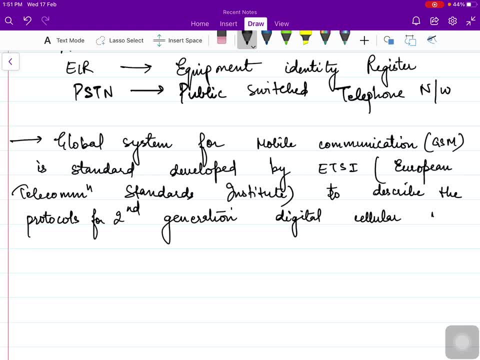 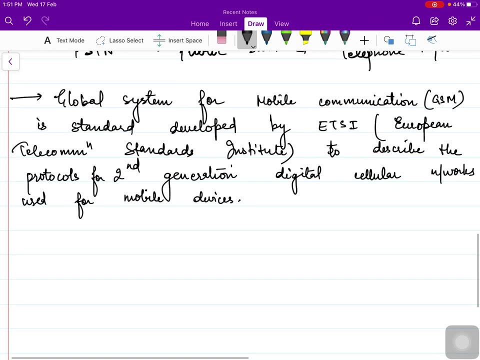 digital cellular networks used for mobile devices, mobile devices. So it was used for, basically, voice transmission and it is a circuit switched system. circuit switched system that divides, that divides- this is an important fact about it, this is an important fact about it- that divides each 200 kilohertz. 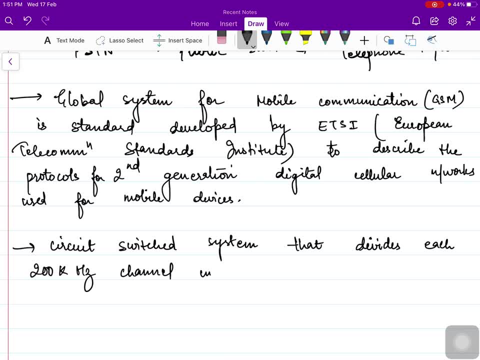 that divides. that divides channel channel into eight slots of 25 kilohertz each. It divides each 200 kHz channel into 8 slots of 25 kHz. So GSM operates on the mobile communication bands. It operates on mobile communication bands 900 megahertz to 1800 megahertz in most parts. 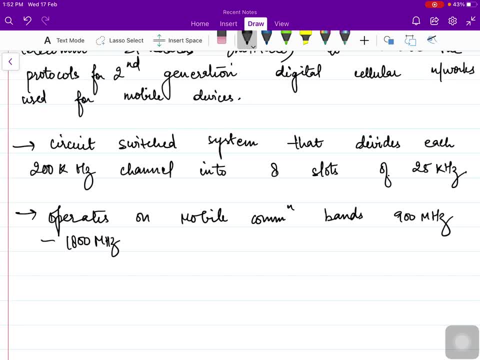 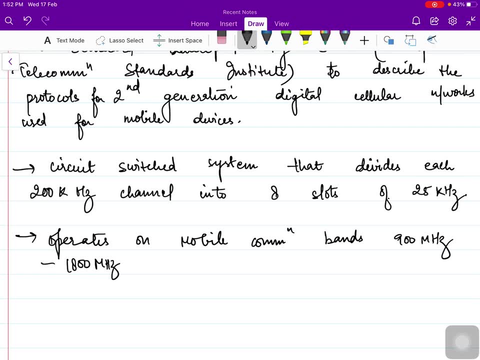 of the world. So we should remember that GSM is a second-generation standard and the second generation was meant for voice transmission. So this is also meant for the same and it defines the protocol because this is a standard. It was developed by ETSI and it is a standard that defines the protocols for second generation. 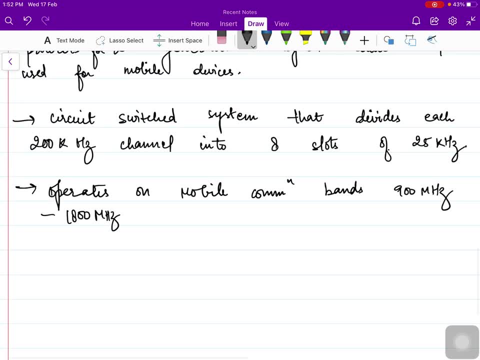 Now it divides. it is a fact about it that it is a circuit switch system and it will divide each 200 kHz channel into 8 slots, and each slot will be of 25 kHz. Okay, so this is one thing. Another thing to remember is the band over which GSM operates. and the next feature, which? 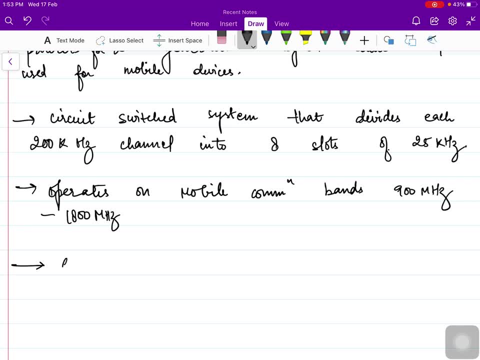 we should remember- is one of the features of second generation- we discussed it there also- that GSM makes use of TDMA technique for spectrum sharing. So for transmitting these signals for spectrum sharing it makes use of TDMA. That is TDMA, That is time division, multiple access technique. 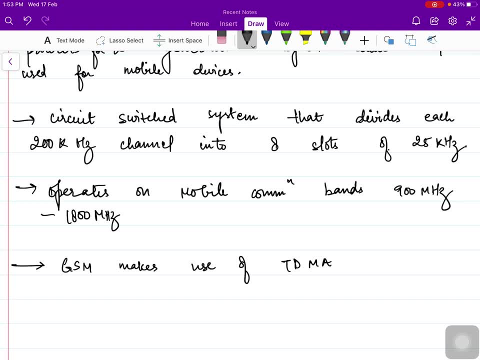 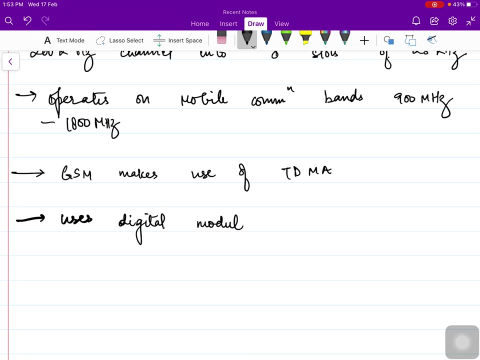 Okay, So these are the major facts and figures about GSM which we should remember. It uses digital modulation scheme. It uses digital modulation scheme, and here data rate increases too. Okay, So these are the major facts and figures about GSM which we should remember. 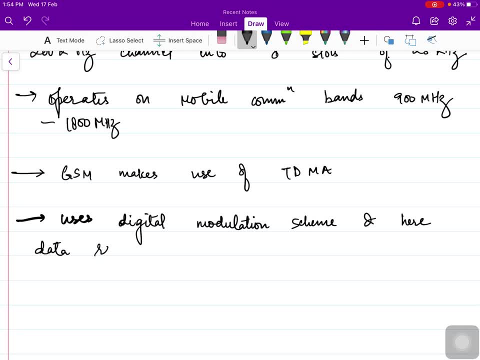 It uses digital modulation scheme. It uses digital modulation scheme, and here data rate increases too. or you can say: data rate is 64 kbps to 120 kbps. So data rate, communication band, what is on what communication band it operates? It is a circuit switch system. 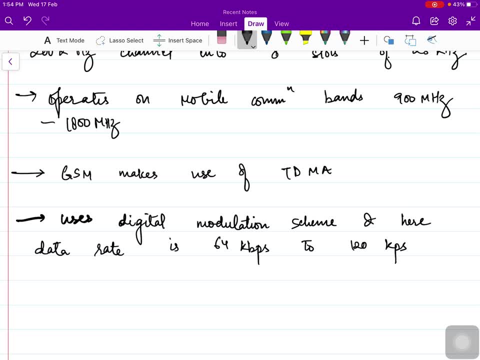 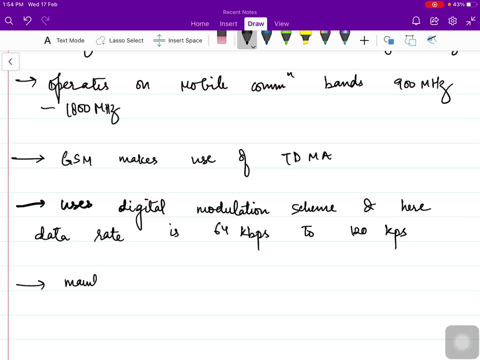 All right, So it makes use of TDMA. These are the main features about GSM, and it is mainly used for voice transmission. Okay, So, these are main points of GSM. Okay, So here is. We have discussed the architecture of GSM. 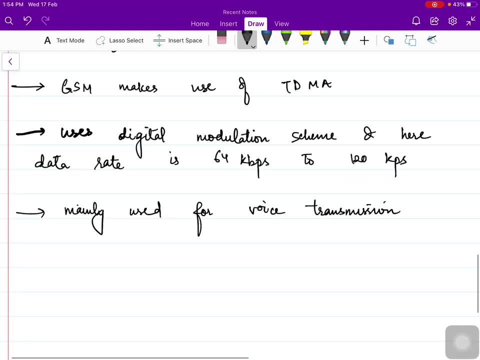 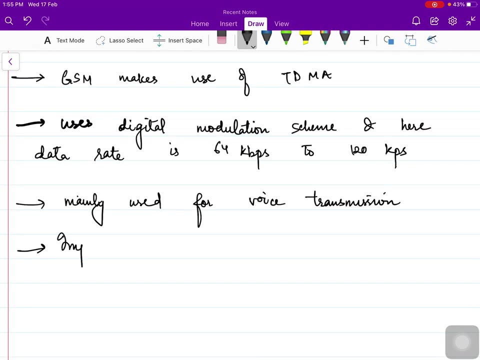 We have discussed the features of GSM. other features are so basically in just if we want to say, are the features of GSN. that was all about the some of the characteristics of GSN. so we have improved spectrum efficiency. improved spectrum efficiency, international roaming, low cost of mobile sets. 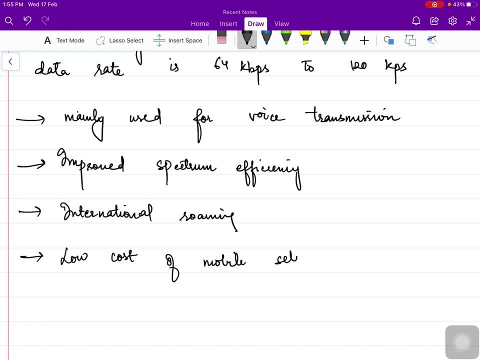 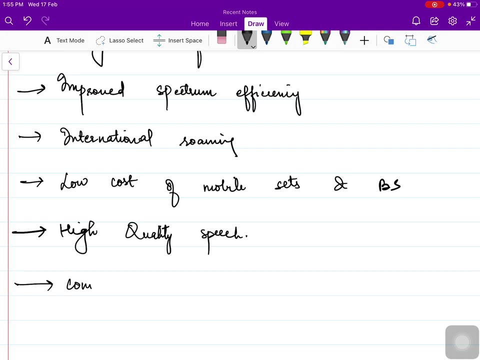 low cost of electronic devices, low cost of digital devices, high-quality speech in GSN, high-quality speech in GSN, compatible with ISDN, compatible with ISDN, compatible with ISDN. and it also supports new service and it also supports new service and it also supports new service: digital network.